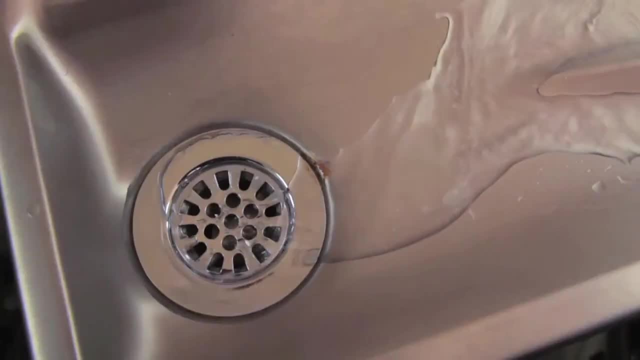 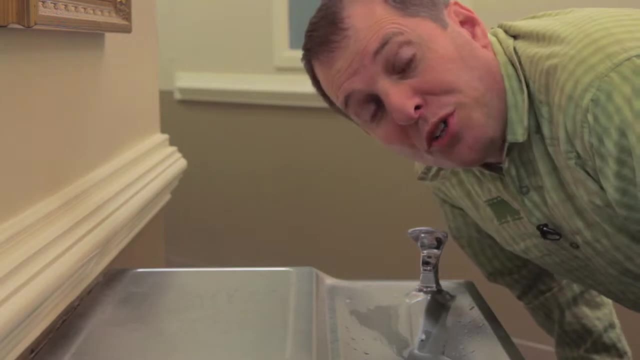 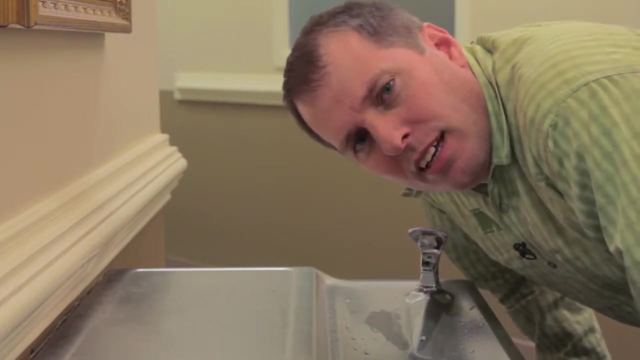 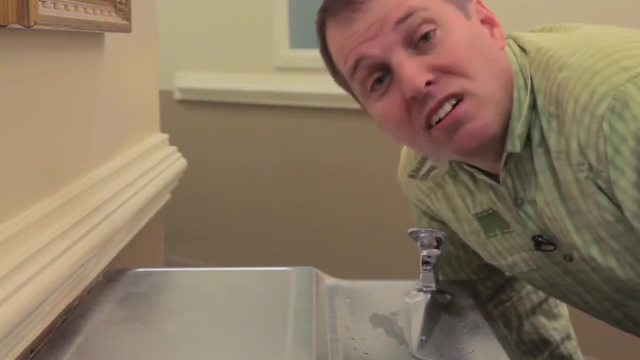 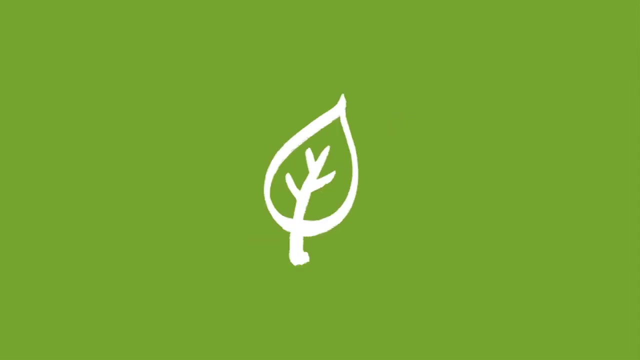 You ever notice how much water you waste when you use the water fountain? What is the impact of this lost water And how much is actually lost, And what would that add up to over the course of the year? Well, we are going to find out, with a little help from Liam. 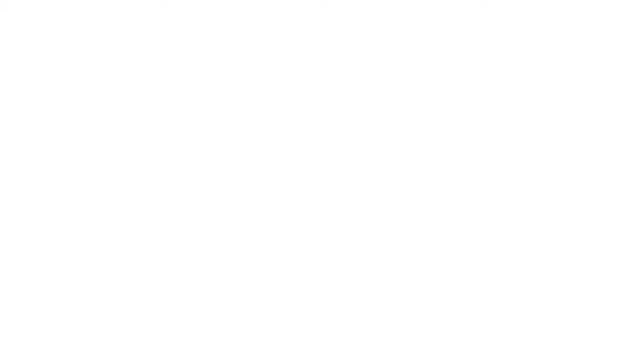 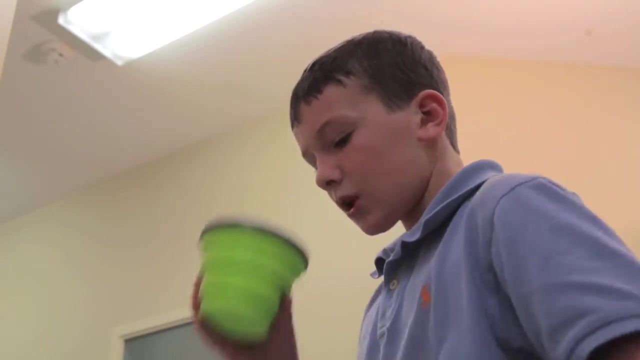 Today we're going to do a little experiment. It will determine how much water is lost during the average water fountain visit, And then we'll demonstrate a simple method to capture this water And finally we'll measure how much we'll save by practicing this method for a whole. 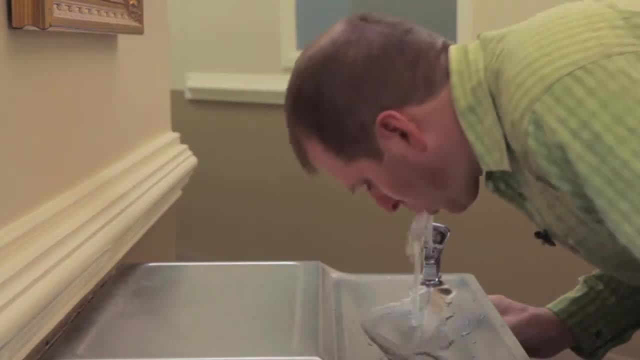 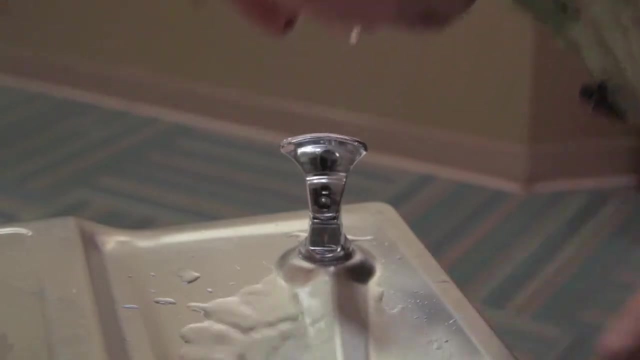 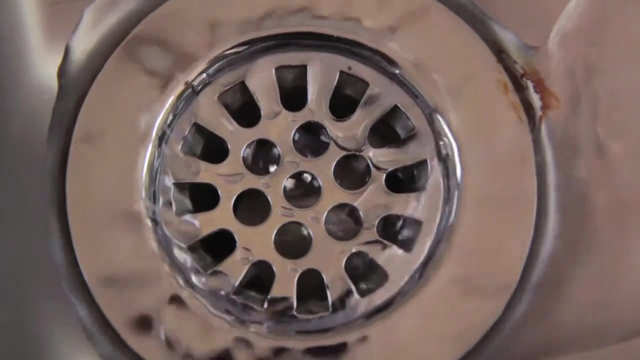 year. Drinking from a water fountain is a good green practice, especially when compared to buying bottled water, Not to mention it's free. This will be an important exercise because it will show that this small trickle of water adds up to a large amount over time. 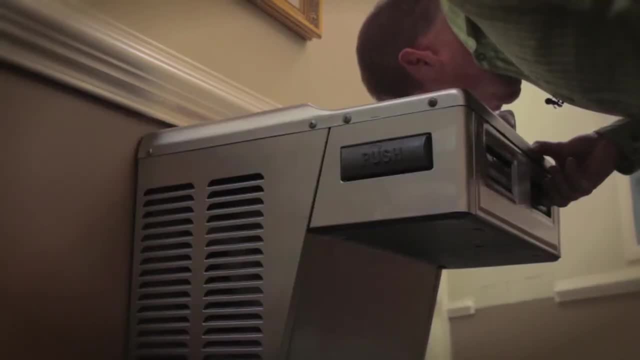 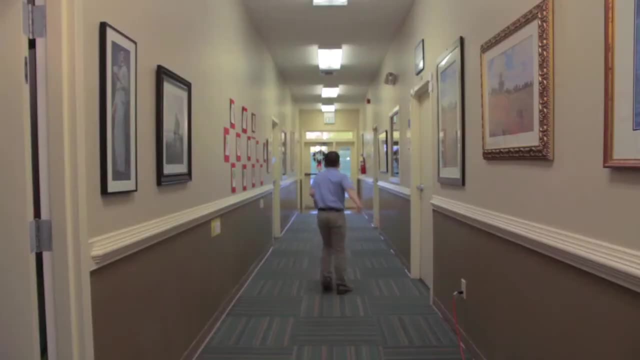 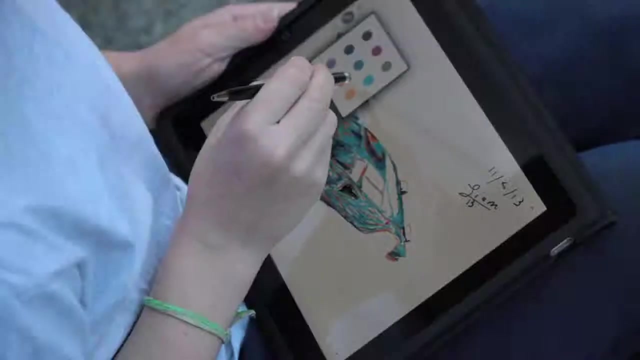 And at the water fountain because the water is chilled. we're also talking about wasted energy, Although we won't try and quantify that. To conduct this experiment, I'm enlisting the help of my friend Liam. He's a big green shorts fan and he's taking personal steps to be more green, like drying on his iPad. 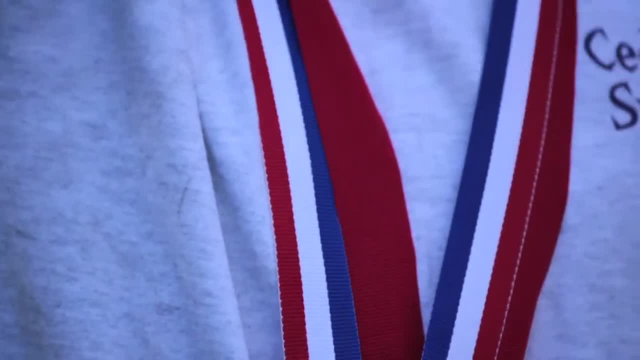 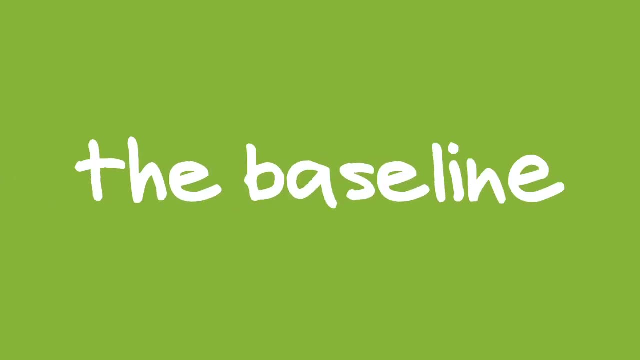 instead of using paper Plus. as a swimmer and a kayaker, Liam cares about water conservation And that's his motivation for helping with this experiment. To get started, we're going to need a baseline. In other words, how long does Liam normally? 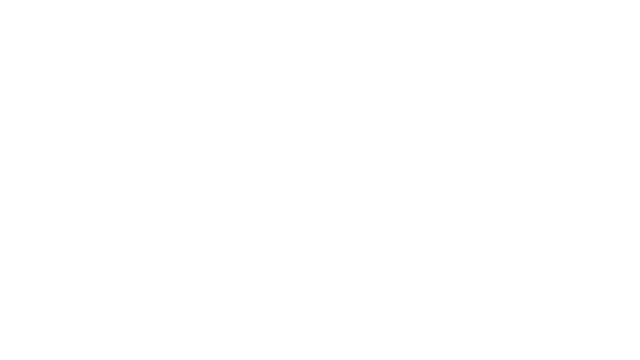 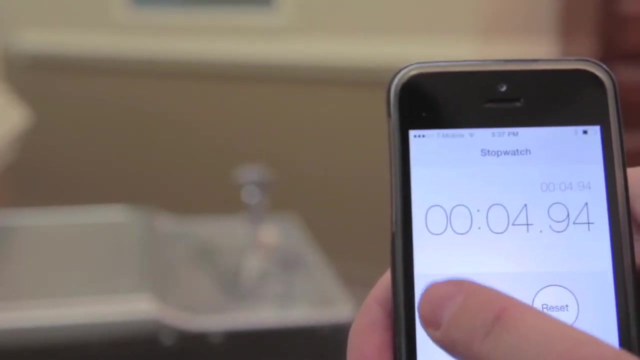 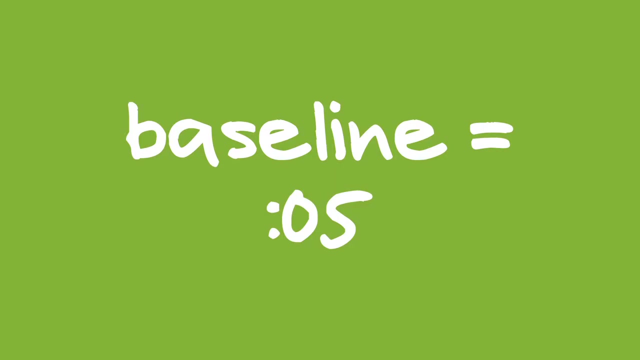 drink from the water fountain. Let's time Liam's drink, So that's nearly five seconds. For the purpose of our experiment, we'll be using a five-second drink at the water fountain. All right, Liam, so we're going to replicate your five-second drink and we're going to 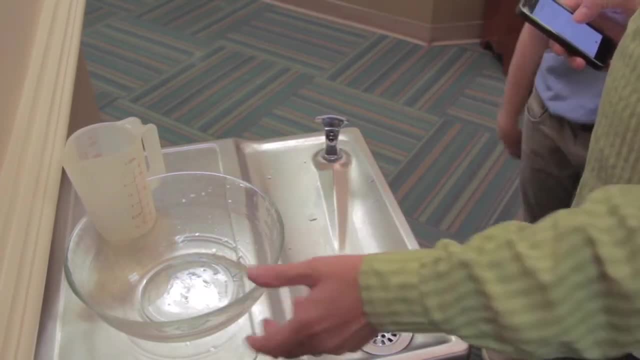 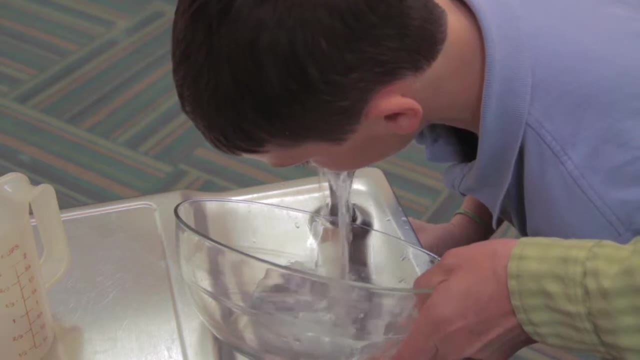 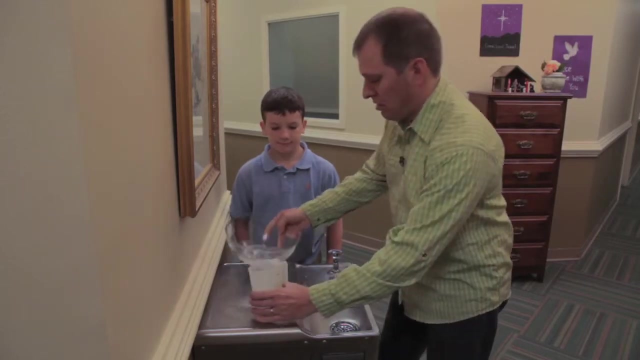 capture how much water is wasted. We're going to measure that. Okay, Ready And go. Okay, One, two, three, four, five, All right. so here's how much water was wasted or would have been wasted, and let's measure that. All right, we're looking at about three-quarters. 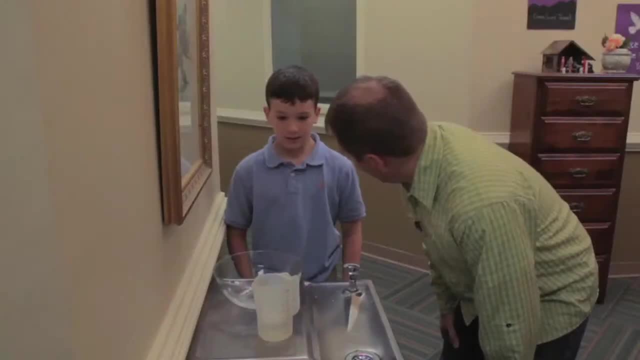 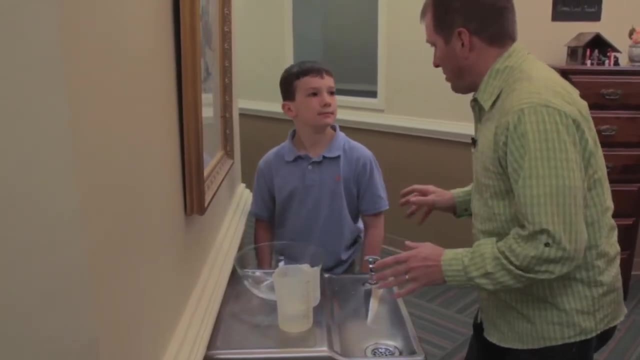 of a cup, a little bit more than that. That's a lot of water. Yeah, Now let's see how much you actually drank. So we're going to do the same thing again. We're going to run the fountain for five seconds, except you're not going to drink any of the 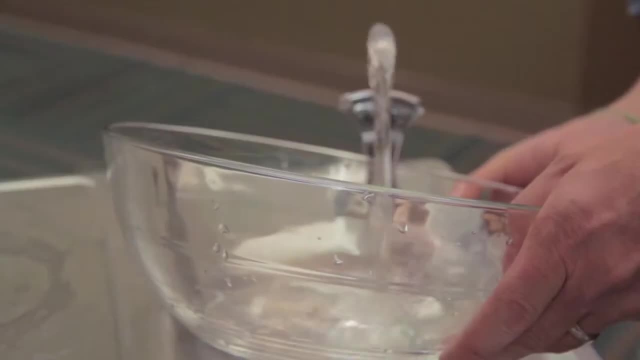 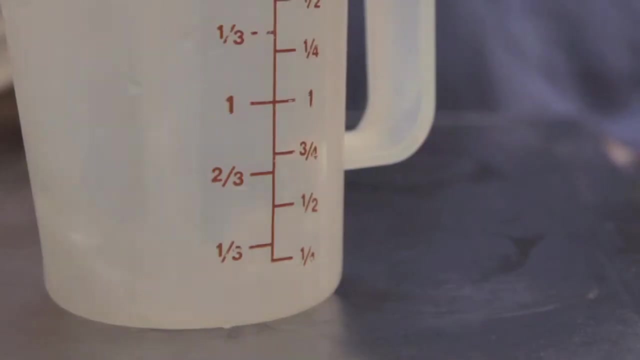 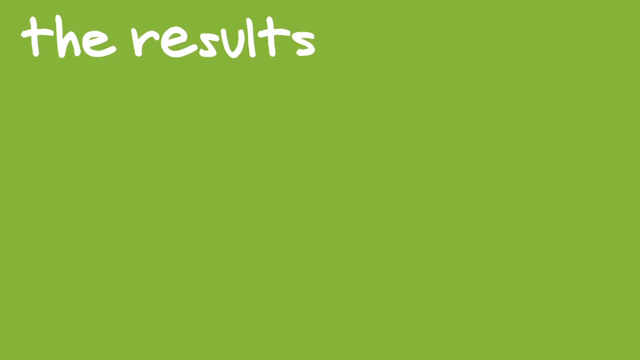 water Ready, Go. Okay, One, two, three, four, Stop. Now let's measure this. Wow, That's just below one cup. And the results: For a five-second drink, one-quarter of a cup of water was consumed. 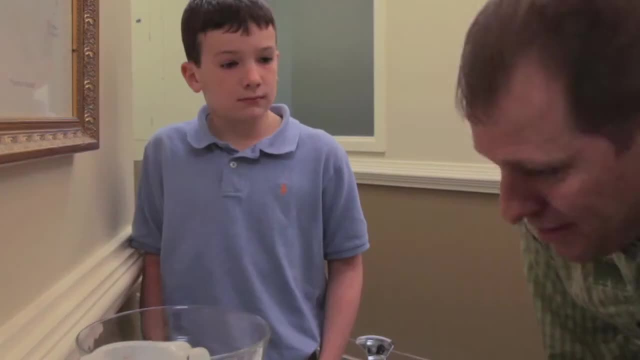 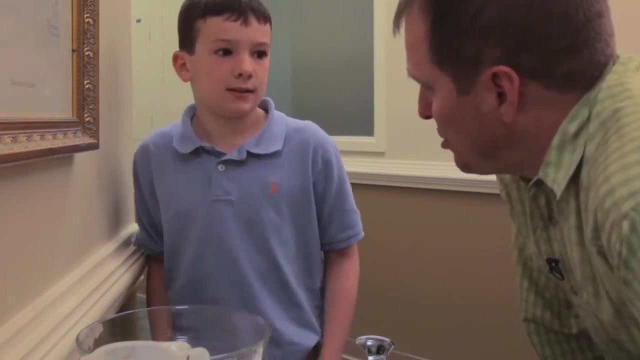 while three-quarters of a cup of water was wasted. So you only really drank a quarter cup of water. That's a lot down the drain, isn't it? Yeah, Do you think you got a solution for that problem? Yep, What's that? 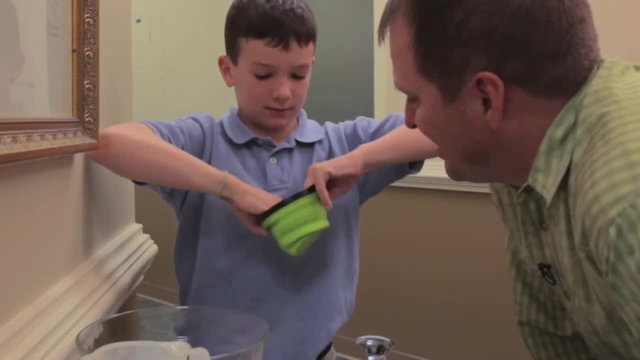 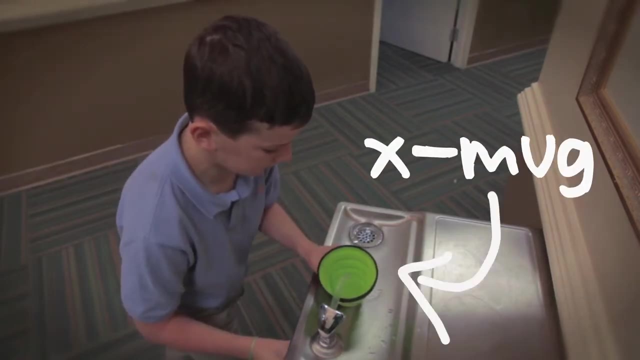 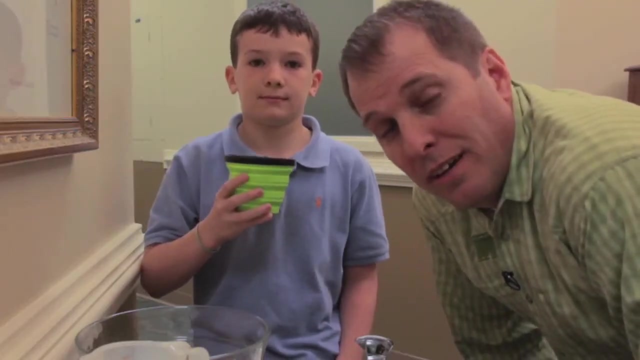 An X-Mug. So here's a little water conservation trick: Every time Liam goes to the water fountain, he's going to bring his X-Mug, He's going to keep it in his backpack and he's going to measure how many times he uses it for a whole year And he's going to mark on his 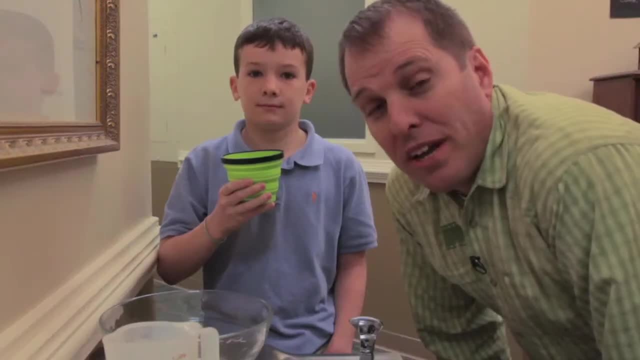 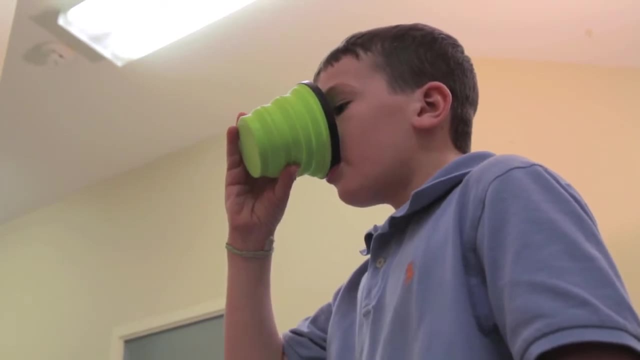 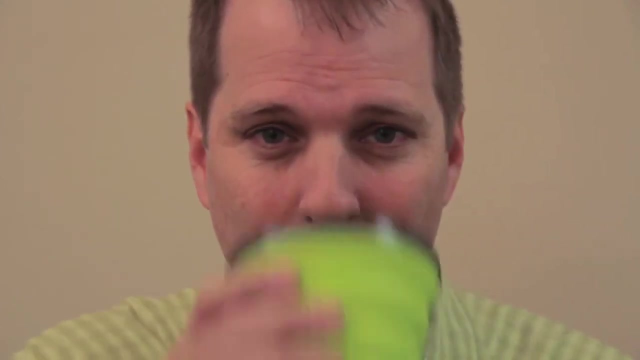 cup every time he does, And we're going to credit each tally mark with three-quarters cups of water. Stay tuned to keep up with Liam's progress And why not join his effort and put the power of multiplication to work. Drinking Like Liam. 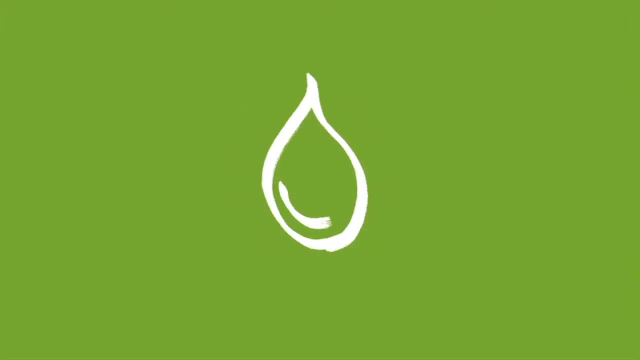 That's just another easy way to be green. As always, our challenge to you: put your green on one leg at a time. Stay connected by becoming a fan of our Facebook page and help spread the green by sharing with your friends. Greenshortscom. 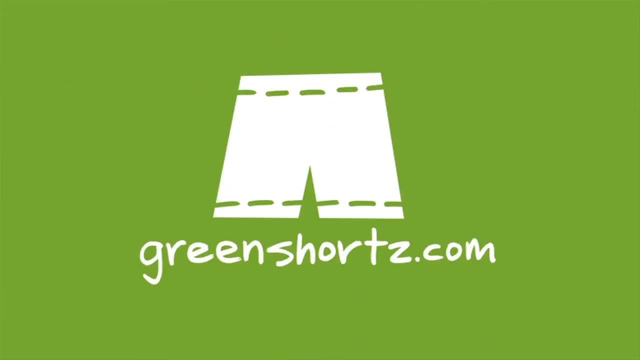 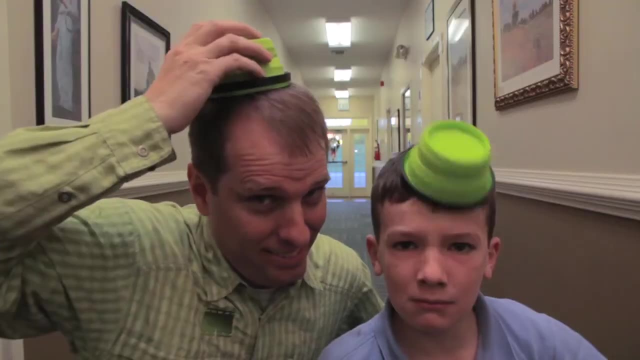 That's shortscom. That's shorts with a Z. Get your X-Mug today. They're all so cute, Little hats, Hats.